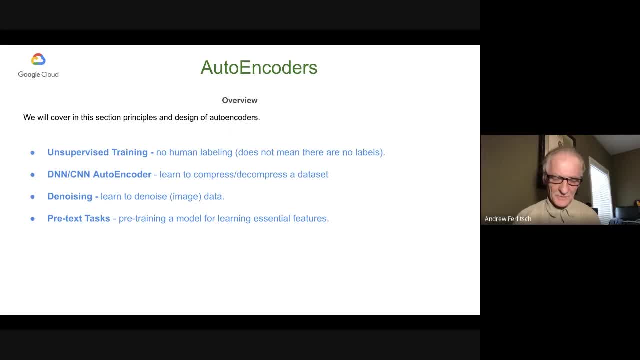 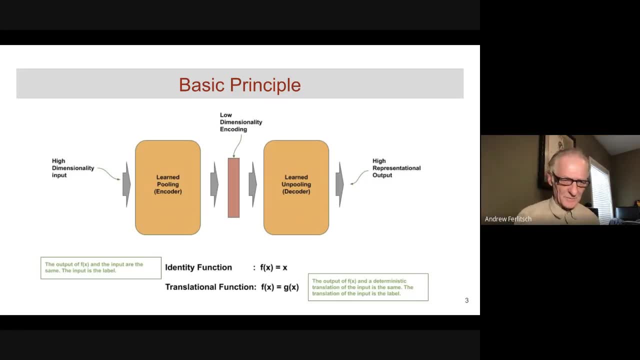 autoencoder for pretext tasks and pre-training of a model to learn essential features. So let's start with the basic principle of an autoencoder. So here at the input, we're going to have some high dimensionality input And for our purpose, just assume that's. 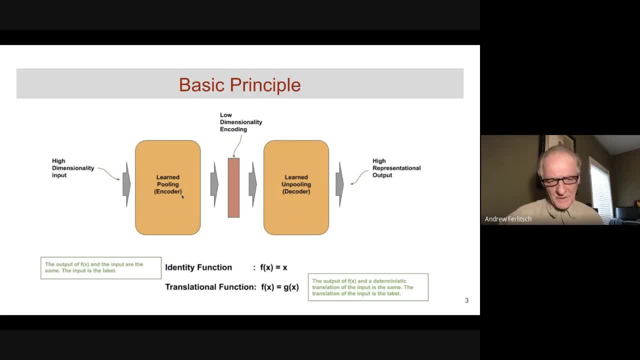 an image And the encoder part is going to, you know, sequentially or progressively reduce the amount of information. And many have seen that chart where it kind of comes down to this, And when you get to a very reduced amount of information it's low dimensionality. we call it the encoding, or in other words, 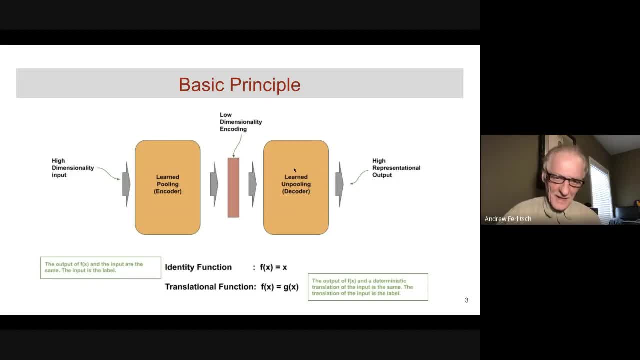 the latent space. Then on the other side of the model, it's all inverted. We're going to learn to unpool the information here. We call it a decoder. It's usually a mirror or a set of mirrors, but it's. 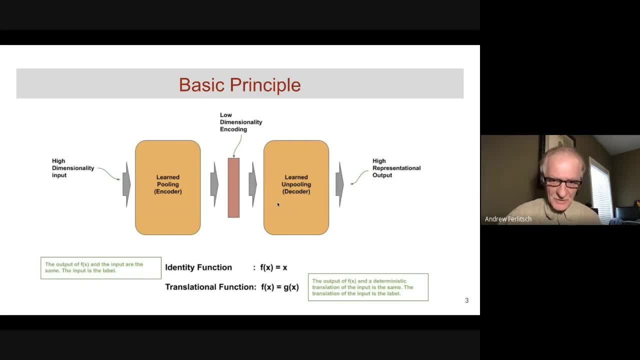 a metric image of this side, just flipped the other direction And it's going to output some high representational output. Now, a couple common things are used for. One is the identity function. The identity function is simply f of x equals x, Or you can say: if I gave the model, 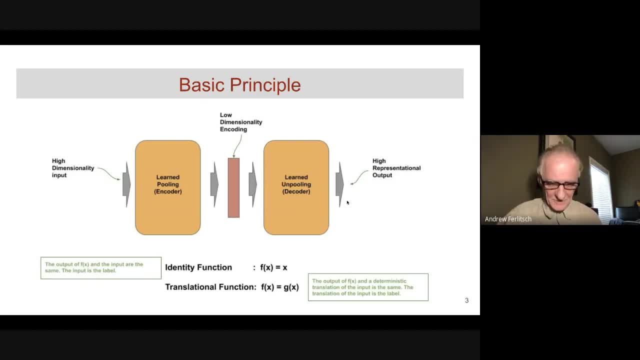 some image x, it would output the identical image, Other forms or functions. we call them translational functions And we call them translational functions And we call them function Given some deterministic function for x, given x, our input. we simply use what we know. 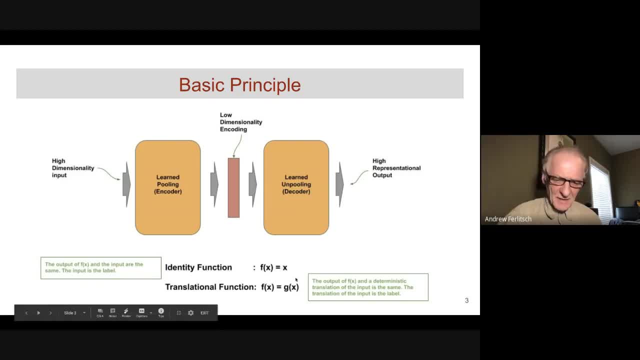 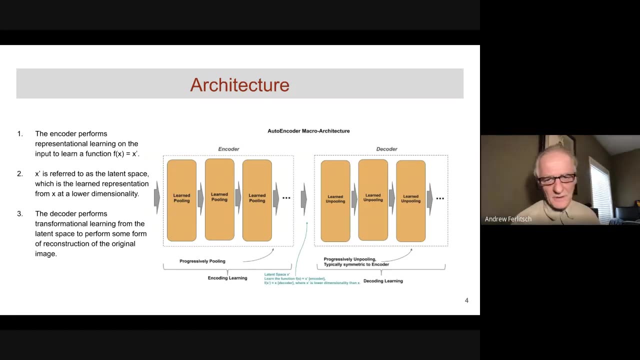 g of x to be the label. So these are examples where there's no human label, but we can use the characteristics of the function to auto-generate the label. So let's look a little bit more at the architecture of auto-encoders. 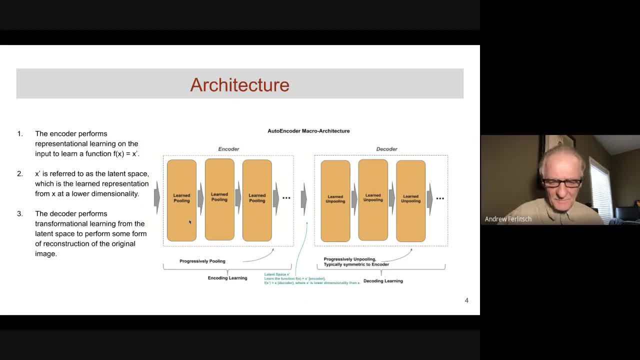 On the encoding side. here you're going to have a sequence of layers where we're going to do what's called learn pool. These layers are going to learn the best way to pool the data And we're going to progressively pool it. That means the data is going to get smaller and smaller and smaller. And then this: 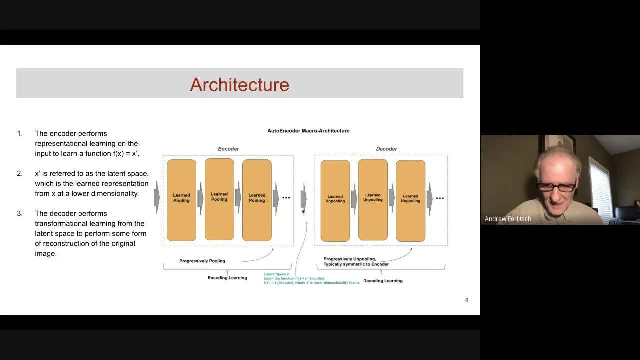 is what we call the encoding learning, And the output of that is what we call the latent space. And then we're going to just do the reverse. We're going to learn We're going to have a sequence of unpooling layers. We're going to learn the best way to unpool. That's going to restore back to the same. 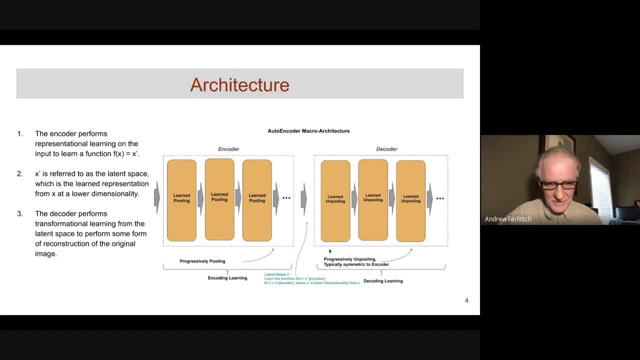 dimensionality And that's typically symmetric to the encoder. So we can also look at it this way: The encoder performs what we call reprisational learning on the input, here to learn the function f of x that generates this latent space. We call x prime, And this latent space is a much lower dimensionality. And then the decoder takes this: 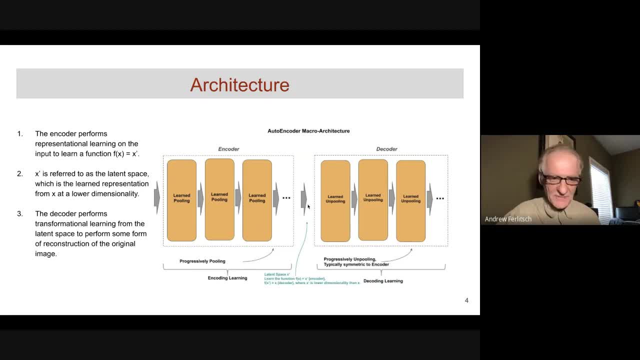 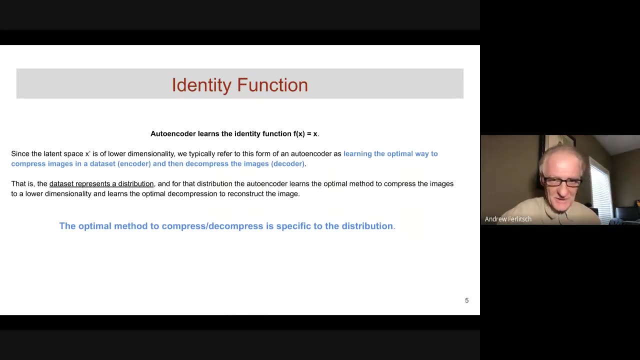 latent space, x prime, and does what's called transformational learning from the latent space to some type of reconstruction of the image into a high dimensional space. So let's start with the identity function. This is usually where everybody is. Everybody starts with an autoencoder And, as I mentioned, it simply means, given some function of x, it outputs x. 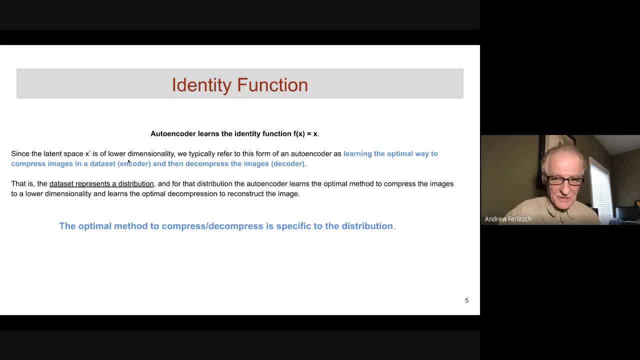 Since the latent space x prime is of low dimensionality, we typically refer to this form of autoencoder as learning the optimal way to compress images in a data set- That's the encoder- And then decompress the images after they've been compressed. 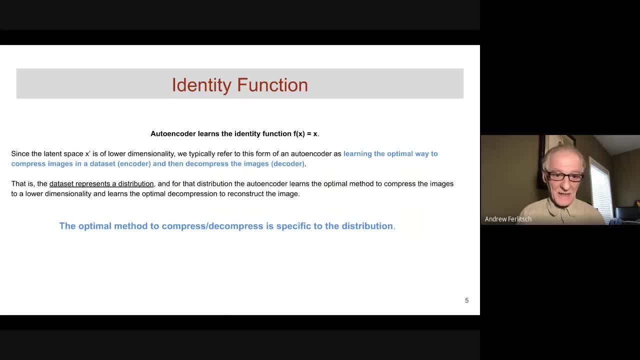 That is this data set. your data set represents a distribution And when it's learning, the autoencoder is learning- is the best way to compress the, say, images for your distribution and then decompress them. What's important to remember is it's specific to the distribution, So if you apply it to a different distribution, you can't expect to have the same level of quality, if any, of the compression and decompression. 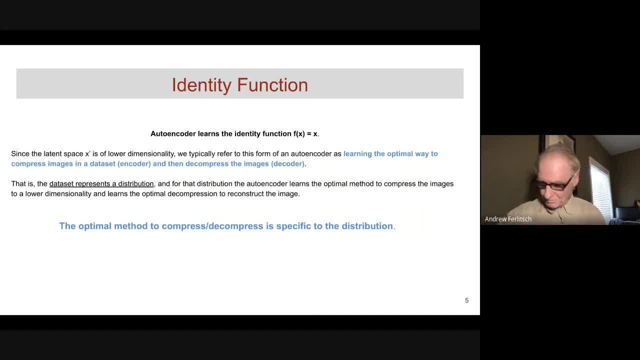 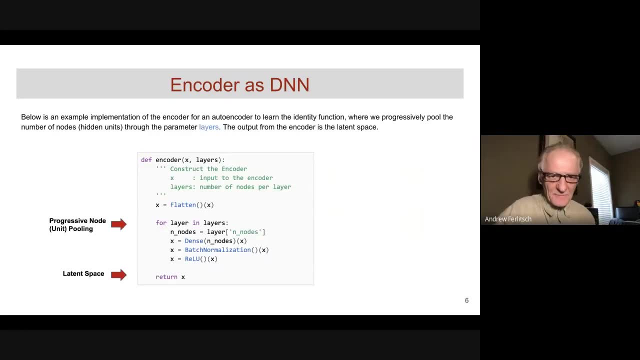 Okay, so this code, a DNN version of an encoder. okay, So what it's going to take is a param. well, first it's going to take the input right, And then this parameter layers and consider this like a list, and it's going to contain a sequence of how many nodes at each layer. 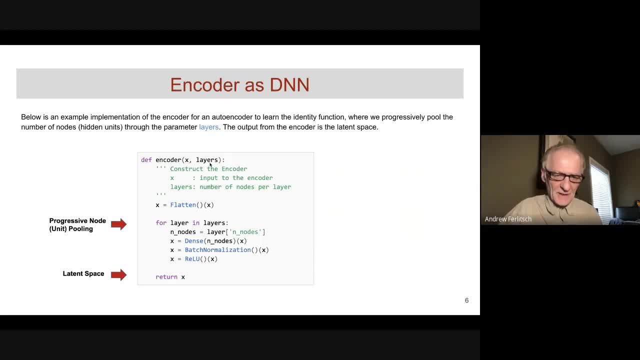 And we're going to presume that that second encoder will actually be: ah, so that second encoder is going to be going to be number one, And then let's take a look at this second encoder. You can see on the screen. Okay, 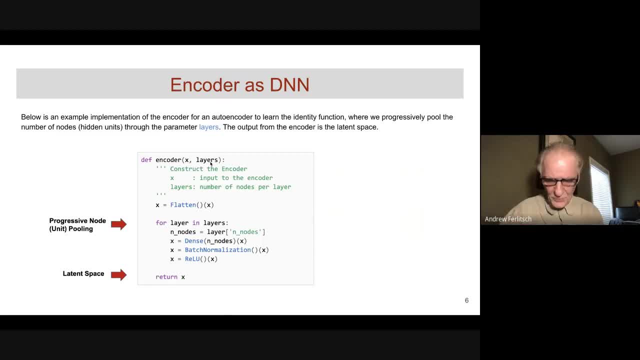 It's going to take a par beautiful one. Okay, because we always progressively pool that that number is going to get smaller. So the first one might be 256, then 128, then 60 floor. We're assuming we're doing this for an image. 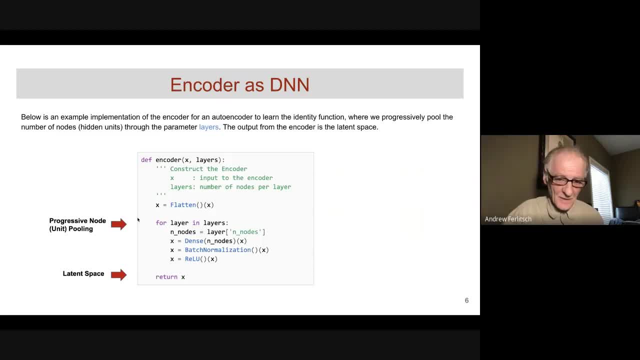 so we're going to go ahead and flatten it into a 1D vector And then we're just going to spin around here and go through this list layer And for whatever nodes we have at that layer, we just create a dense layer. 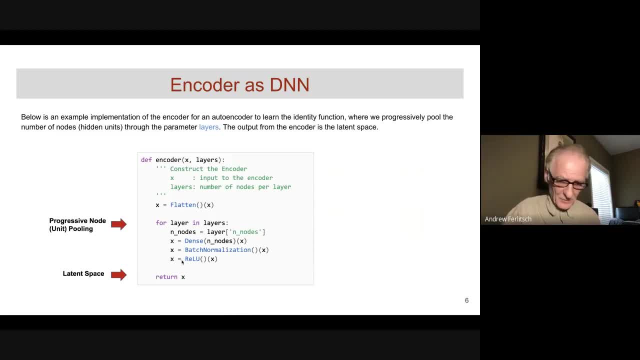 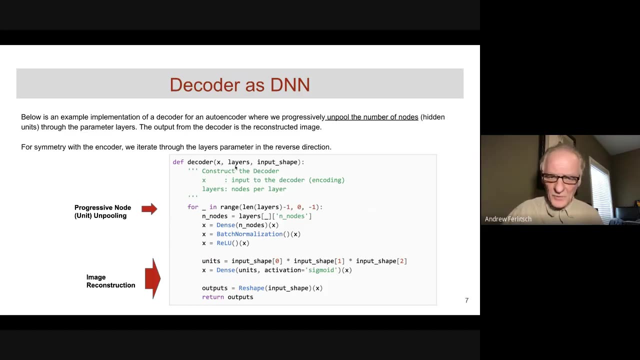 Then the output of that, the final output of all that progressive pooling, is our latent space. So writing an encoder for a DNN is really straightforward. The decoder we just want to- in a sense we really want to take this layers, the same layers list that we used for the encoder. 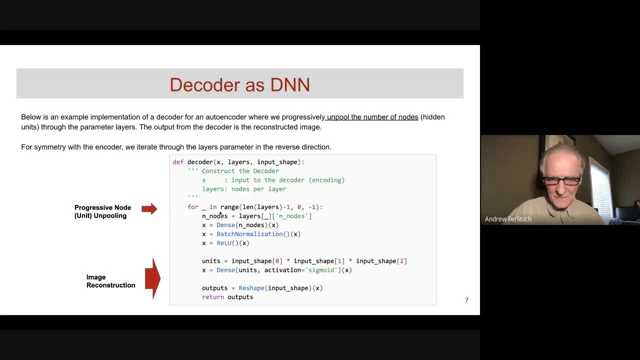 but go in the reverse direction. So you can see, I'm doing that here in the for loop. I'm just going in the reverse direction And I'm recreating all these dense layers to do progressive unpooling. So, given our example of 256,. 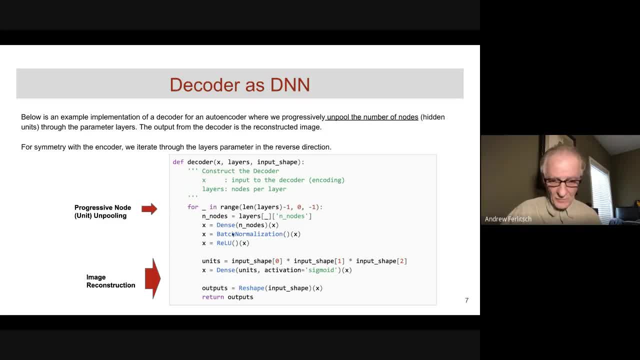 128, 64,. you'd have 64, 128 to 56.. Finally, when we're done with all that, we want to make a final layer OK, and that final layer is we're going to want to reshape our output. 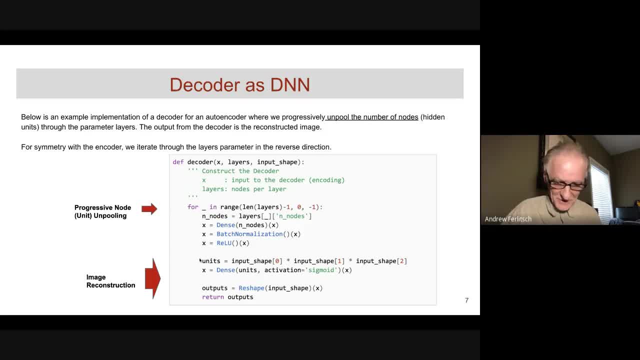 because this is the identity function And some of you just may just notice this isn't indented. It should be OK. So, first, the number of units is going to be equal to whatever the input shape was To the model. OK, that's how many units we want, or nodes. 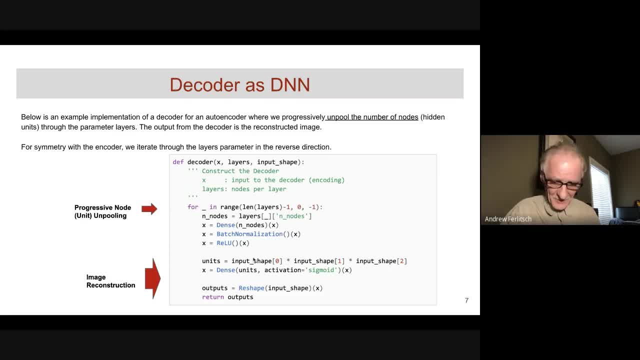 OK, each one of those. OK, so those are our pixel values. We want to map them. These are real values between zero and one. Remember our input was normalized between zero and one. So the activation function that that's going to squash. 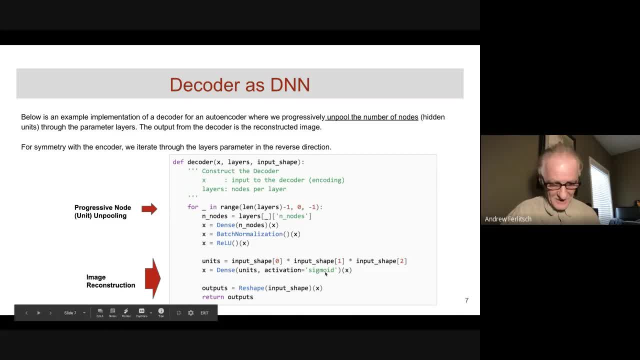 all the outputs between zero and one is a sigmoid, And that's why we use a sigmoid. And then, finally, we're going to reshape that output into that image shape. So that's our image reconstruction. So here is an example of me training one. 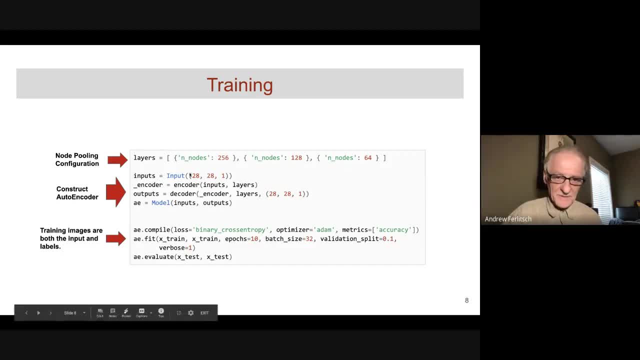 OK, this was for minced, So you can see my layers were 256,, 128,, 64. So I create an input object. I then create the encoder. given the inputs and the layers, I get my encoder output and then I create the decoder. 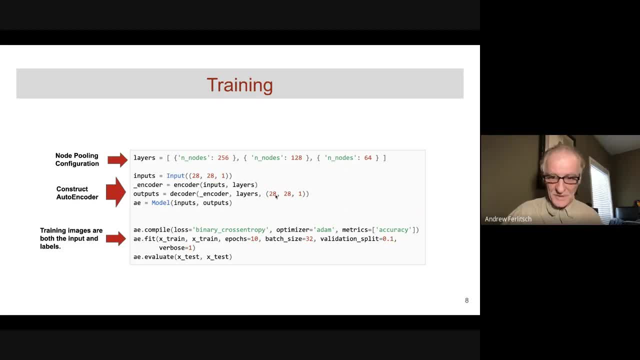 giving the output here as the input here, the layers, of course, and then the input shape. OK, then I just put the model together. That's my auto encoder. I'm going to compile it because I'm using sigmoids. 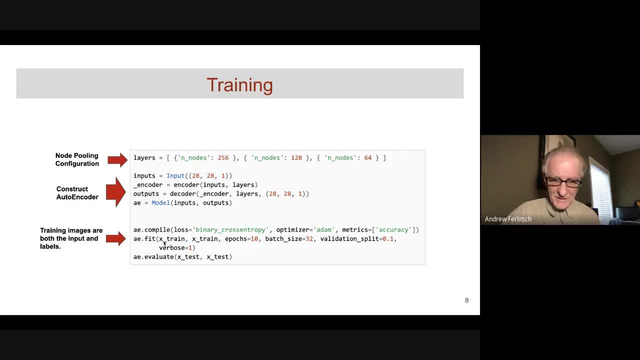 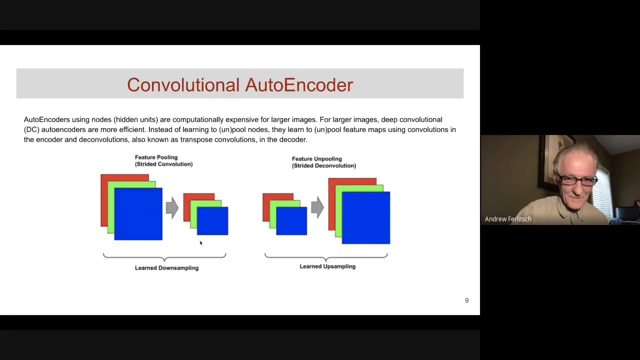 That's going to be a binary cross entropy, And then when I train it. really the only thing here that's important is I use the images X train for both the, for both the training data and the label. OK, so let's now move on. 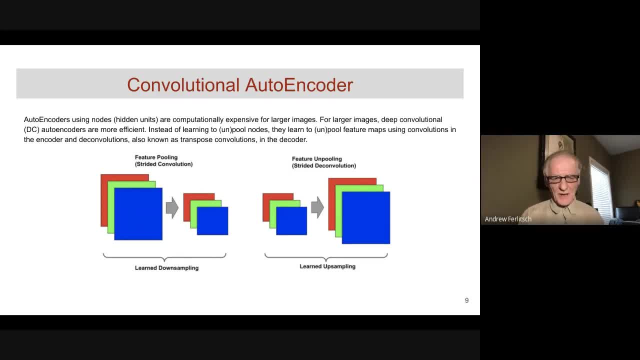 To convolutional auto encoders. So auto encoders that use nodes or hidden units are actually computationally expensive for larger images. They're just not practical. So for larger images we use deep convolutional auto encoders and they're much, much more efficient. 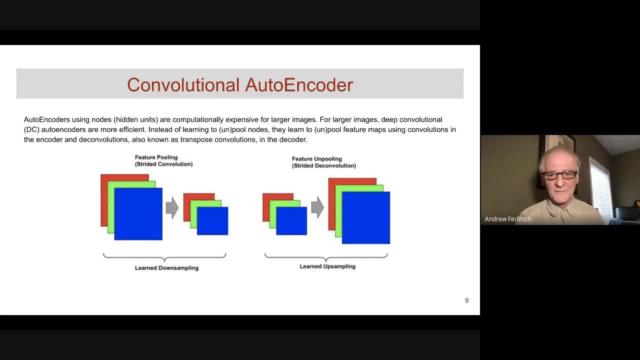 So, instead of learning to pull and unpool nodes, they learn to pull and unpool feature maps using convolutions in the encoder, and deconvolution is also known as transposed convolutions in decoder. Now, at this point, many of you might just not know. 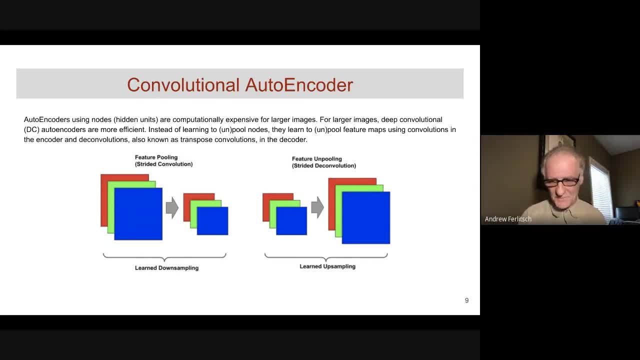 what's a deconvolution or a transposed convolution? So I'm going to give you a quick explanation about the differences. So by now you would be familiar with the idea of feature pooling. in a convolution, That is when we set the stride to two, whatever we output in feature maps. 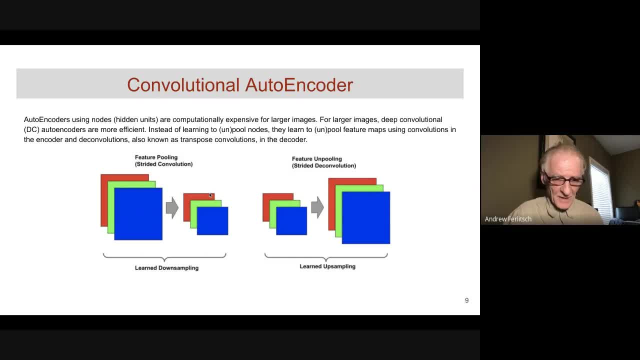 is going to be one half the height and one half the width. In effect, we're learning to downsize. So, for example, a deconvolution does the exact opposite. So if you start with these as the feature maps and you set the stride of two, 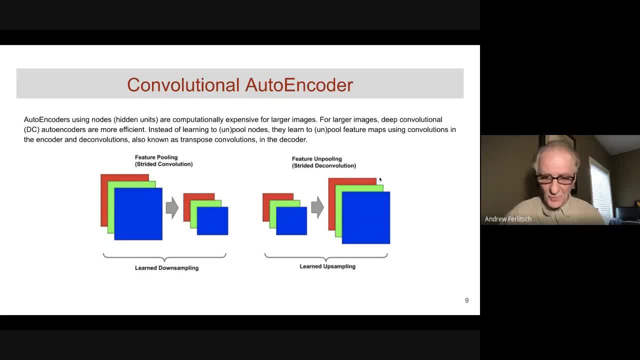 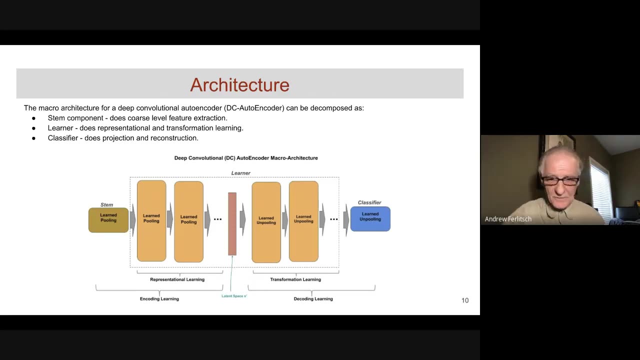 it's going to output feature maps that are two times as high, two times as wide. So what it's doing is learning the best way to upsample. That's the only difference between a convolution and a deconvolution. OK, so let's look at the architecture for a deep, convolutional auto encoder. 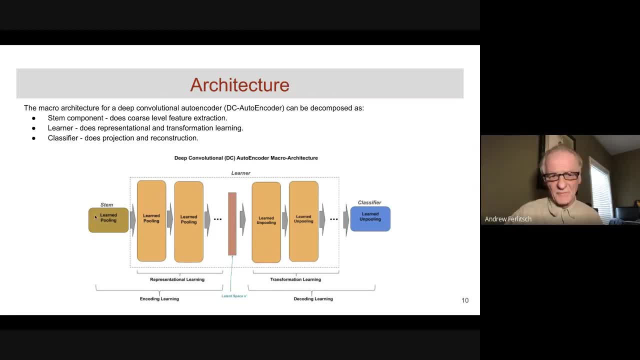 So you have your initial stem here. that's going to do a course level feature extraction. OK, then the learner part is going to effectively have your encoder, your decoder, your latent space. OK, and this is where you're doing your repositional learning into the latent space. 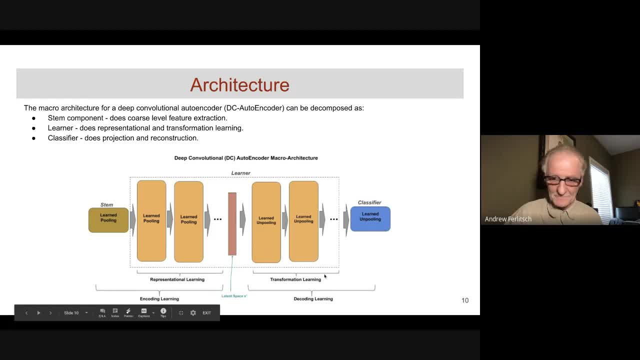 And then the decoder is where you do your transformational learning, And then, finally, you have a classifier, which is the learn task that you're going to do. So even the stem is part of that. The classifier is part of the learn pooling and the classifier is part of the learn unpooling. 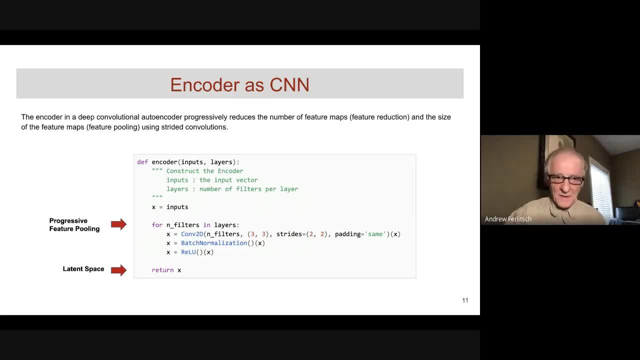 So let's go ahead and write one of these, OK, so here we're going to do something similar in layers, except for layers, instead of the number of nodes, it's the number of filters, And again it's going to be a list where it's going to be progressively get smaller. 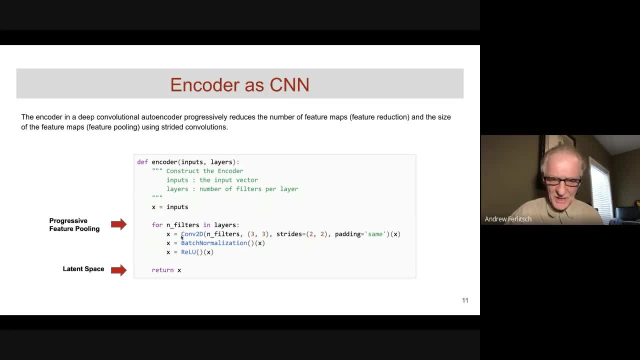 So we just spin through the list And each time we create a convolutional layer of that many filters And of course it's strided, So we have feature pooling, So it's getting less, less, less, less, OK, and then finally the output of that would be our latent space. 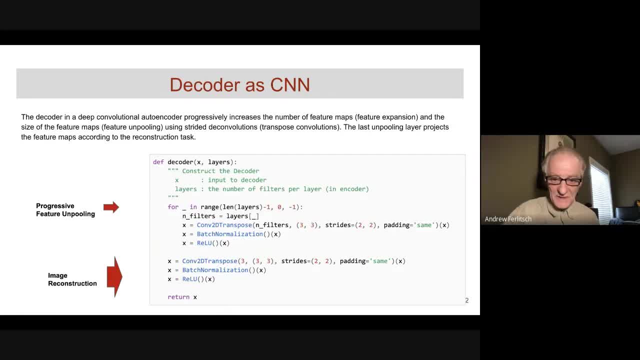 So let's look at the decoder Again, it's going to do the exact opposite. OK, so you're going to give it that layers list. You're going to go through it in the reverse direction, reconstructing from the lowest value to the highest value. OK, so you're going to give it that layers list. You're going to go through it in the reverse direction, reconstructing from the lowest value to the highest value. OK, so you're going to give it that layers list. You're going to go through it in the reverse direction, reconstructing from the lowest value to the highest value. 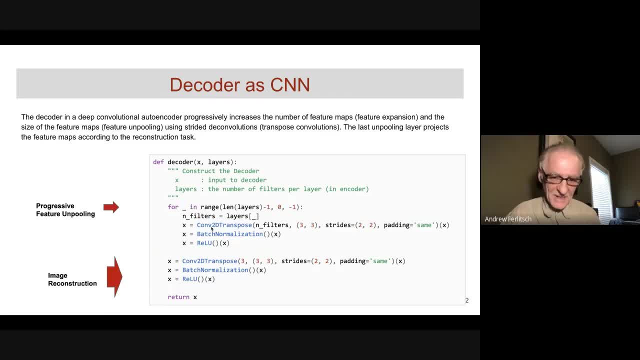 OK, but now we're going to do a deconvolution. in this case is called Conv2d transpose in Keras, And of course it's a strided deconvolution. So the featuremaps coming out there are going to be double in size. 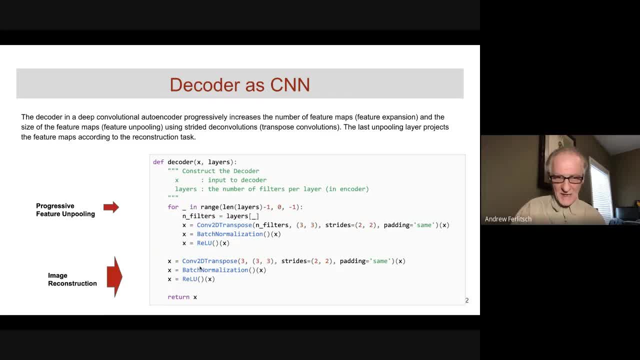 Then the last step is: is we need to reshape or reshape that output to match the input? Then the last step is: is we need to reshape or reshape that output to match the input? So here, the input being, let's say, you know was RGB- 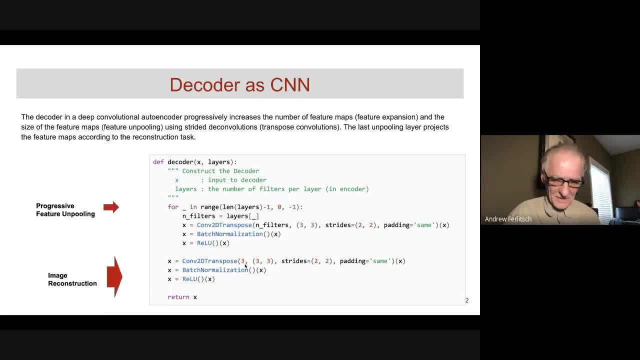 So here, the input being, let's say, you know, was RGB. So here, the input being, let's say, you know, was RGB, to have three channels, and we're going to do our final deconvolution to learn to shape it to the. 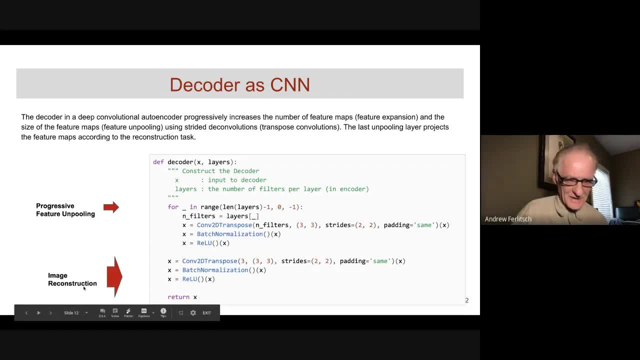 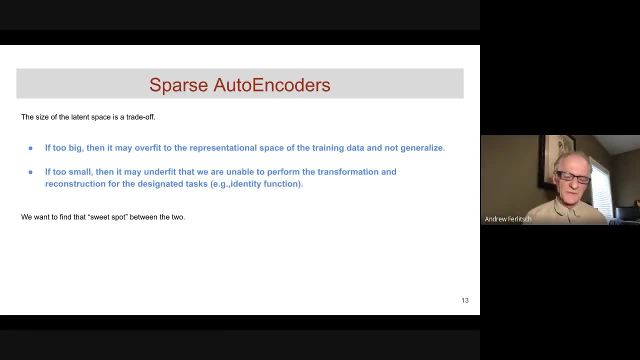 output And then we're going to return that. So that's our image reconstruction. Now, what size of latent space do we use? Well, you know, you might think, well, the bigger it is, the more likely I can do learn the identity function and the better compression and more. 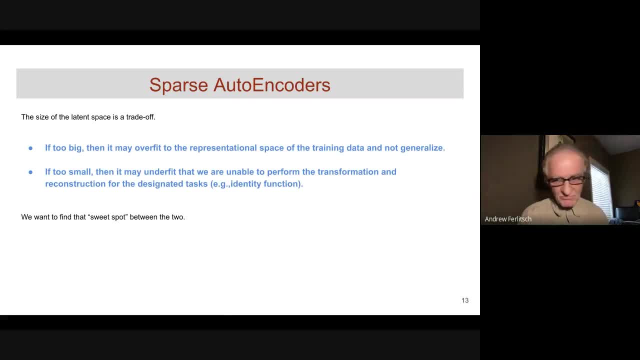 liable my compression and decompression would be? Maybe not, because if it's too big it may overfit to the reprisational space of the training data. That is, if it's too big it may have overcapacity and then overfit to not the training data itself but the training data's reprisational 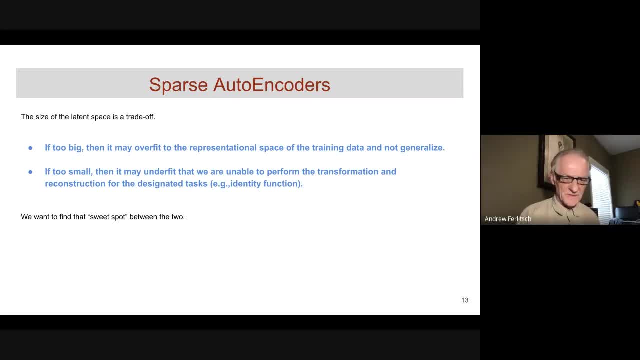 space. On the other hand, if it's too big, it may overcapacity and then overfit to the training data. If it's too small, it may underfit and we won't be able to do that. on the other side, the 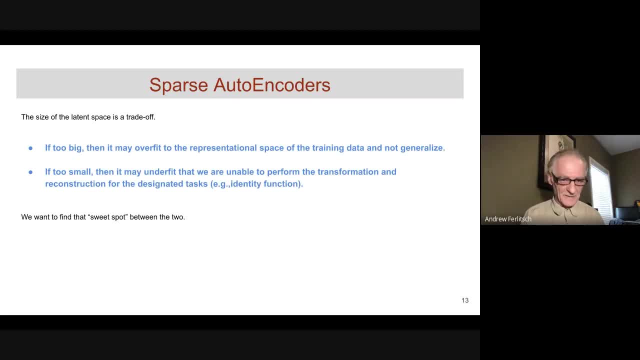 transformation and reconstruction for the designated task, like the identity function. So what we want to find is the sweet spot between the two. So one way we do this- and we refer to it as a sparse autoencoder- is we're going to add a. 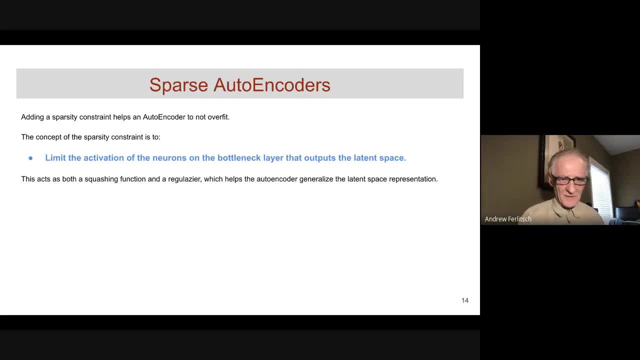 sparsity constraint to not overfit, And the concept of a sparsity constraint is to limit the amount of space that we have in the training data. So we're going to add a sparsity constraint to limit the activation of neurons on the bottleneck layer that outputs the latent. 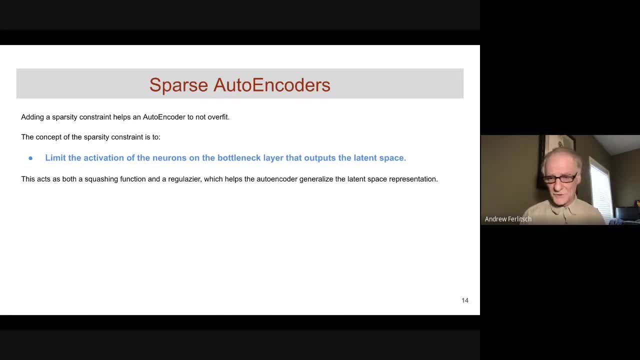 space. So think of again the convolutional autoencoder. You get to that last convolutional layer and it's output. we're going to flatten. That's our latent space. But the activation function here, in addition to being a ReLU, we want to do some further squashing of those values. 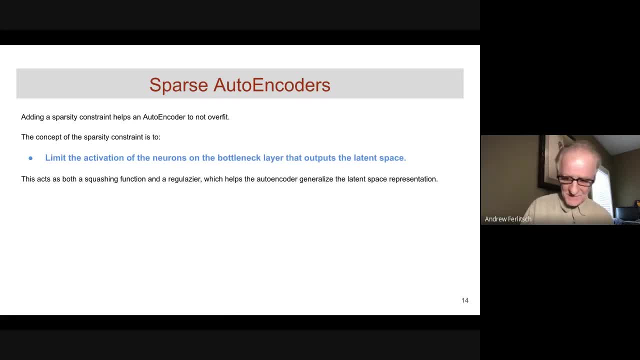 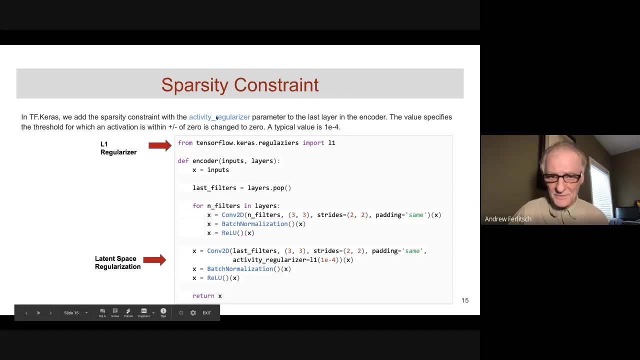 as it acts as a regularizer. So in Keras that's referred to as the activity regularizer. The word activity here really is referring to the activation. We're applying a regularizer to the activation And we're going to do it as the last parent layer in the encoder And the value is going to specify the threshold. 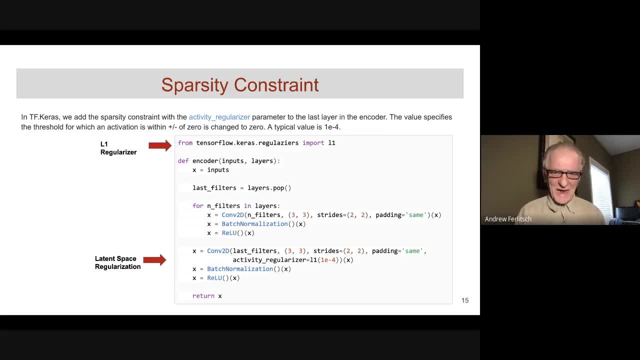 plus or minus around zero, that we're going to change back to zero. So it's what it's saying is, these tiny, tiny layers are going to change back to zero And we're going to change back to zero. So if we have these little values that make or just don't contribute much, we're just going to treat. 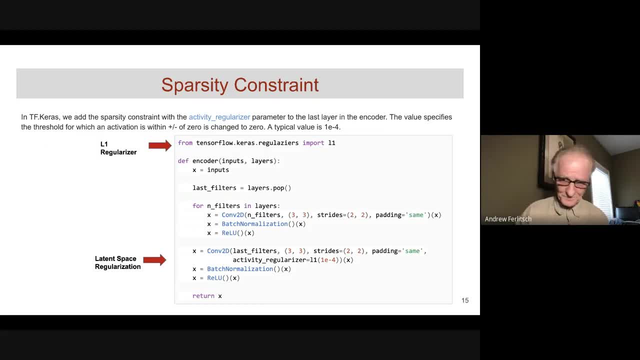 all of them as zeros And that's like saying no signal And that adds a little bit of noise or regularization to our model. And a typical value used is like one to the power, yeah, one to E minus four. So let's go ahead and write an encoder that does a sparsity constraint, Okay Well. 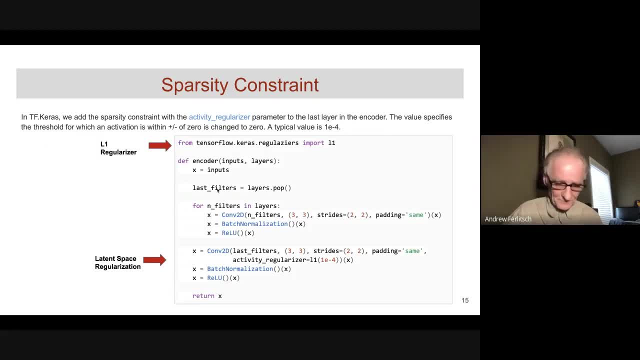 this time we want to set aside The last layer, So I'm just going to set it aside, Then all the remaining layers. of course I do my normal convolutions And then when I get to the last one, that's going to output that latent. 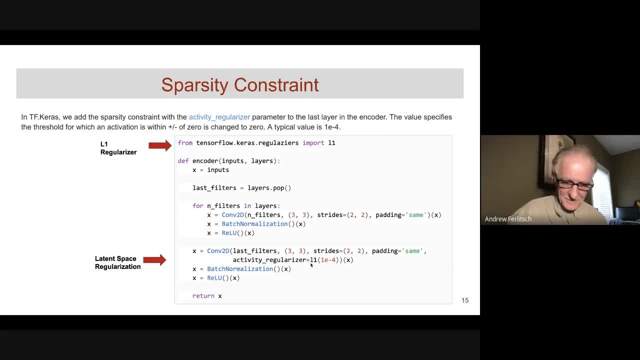 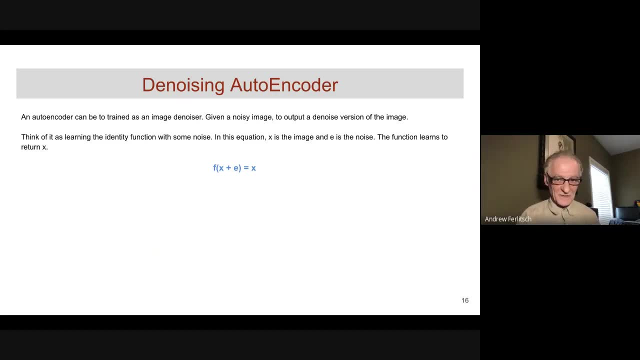 space, I'm going to add the activity regularizer. Okay, So up to now we've only talked about the identity function. You may ask: what else can we do with an autoencoder? Well, the next thing people tend to learn to do is what we call a denoiser, And that's what we're going to do. So we're going. 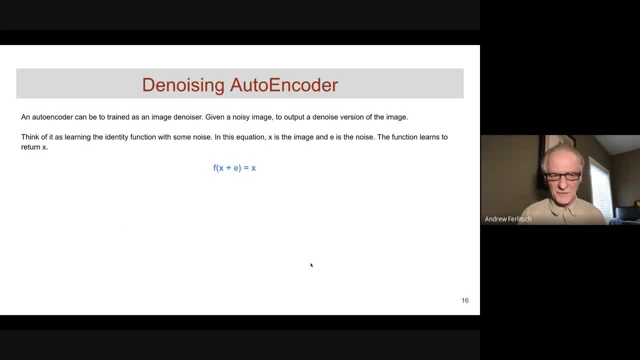 to use an autoencoder And the idea is that it's an autoencoder that learns to be an image denoiser. So we can say it like this: given a noisy image, to output a denoise version of the image. A simple way of thinking of it is thinking that you have some noise here E And what you're. 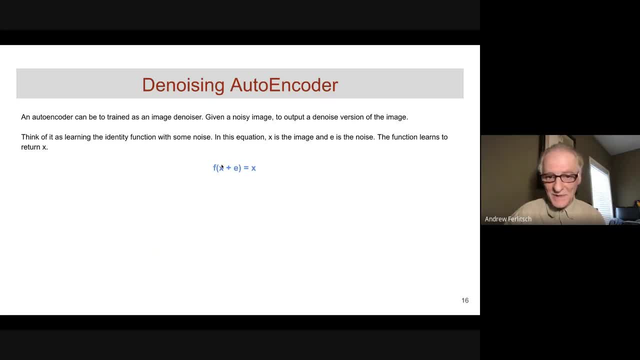 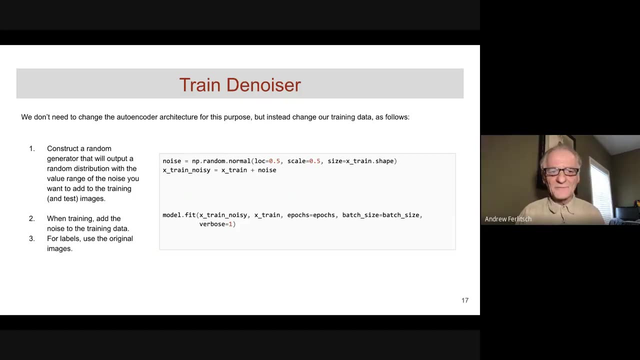 learning is you have a function that takes an image plus its noise and it outputs that image. So that's the function we're going to learn in a denoising autoencoder. So it's really easy to do one. You don't have to change the autoencoder to. 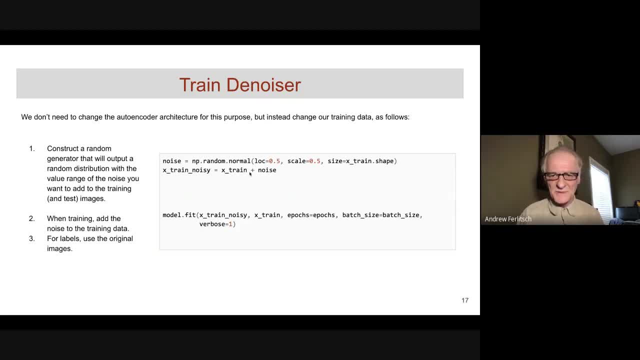 do this. You can use your existing autoencoder. What you do instead is you change your training data. Okay, So in this example, I'm just going to get a random distribution of some tiny values. That's going to be my noise, And then what I'm going to do is I'm going to apply that noise to 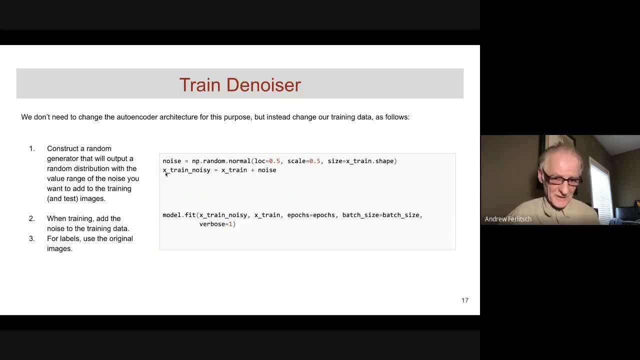 my training set to get a noise. And then I'm going to apply that noise to my training set to get a noisy version of the training set. Remember, these are numpy arrays, So this operation gets broadcasted across this entire training data. And now, when I train, the noisy training data now: 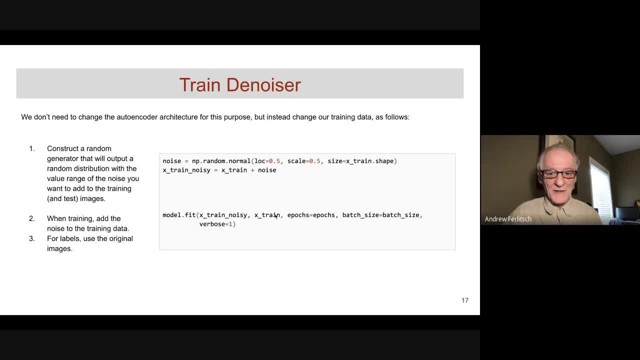 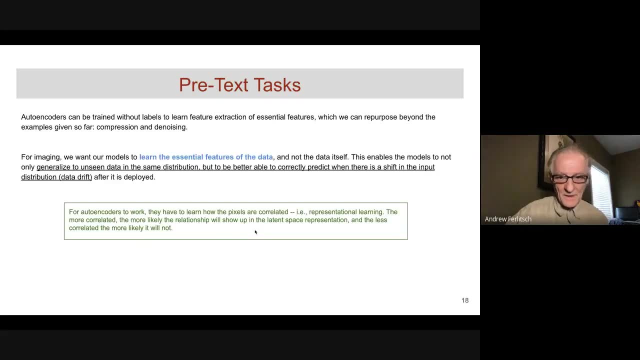 becomes my input, That's that X plus E And my output is the original training data And that's training an image denoiser. So we'll wrap up here with pretext tasks So autoencoders can be trained without labels to learn feature extraction of essential features. 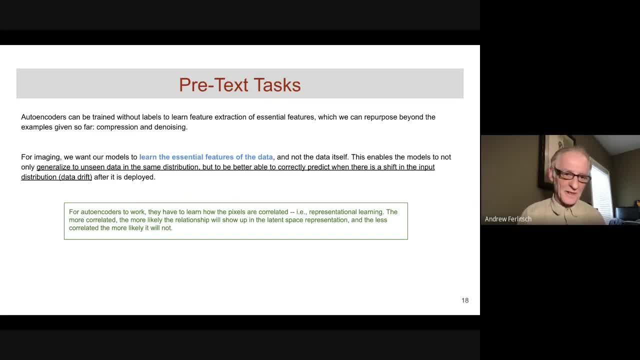 Okay, And we can repurpose this ability beyond things like compression and denoising, And one of the ways we do it is we actually use pretext tasks to help train, initially, do some pre-training of a model that we're going to train in a supervised fashion, And our 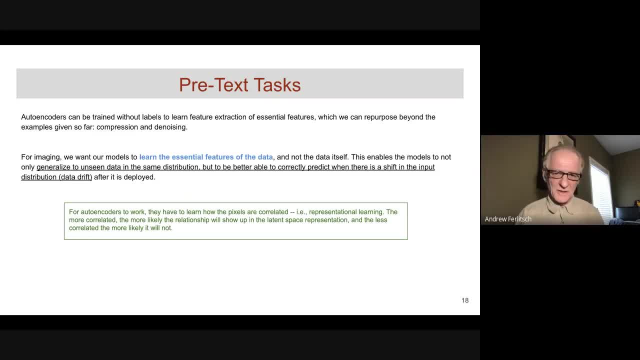 purpose is to train the model in a supervised fashion, And we're going to train the model in a supervised fashion. And our purpose is we want to learn the essential features of the data, And we're going to use an autoencoder to do that. And by doing so, the model not only, do we want it to. 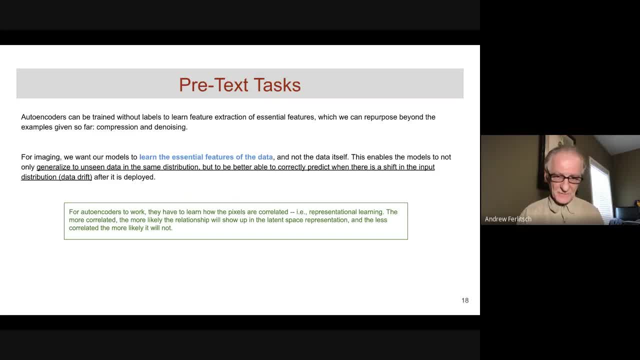 generalize to unseen data in the same distribution. but if we're really just learning the essential features, then in principle it should be able to correctly predict when there's a small shift in the input distribution that we call data drift, after it's employed. 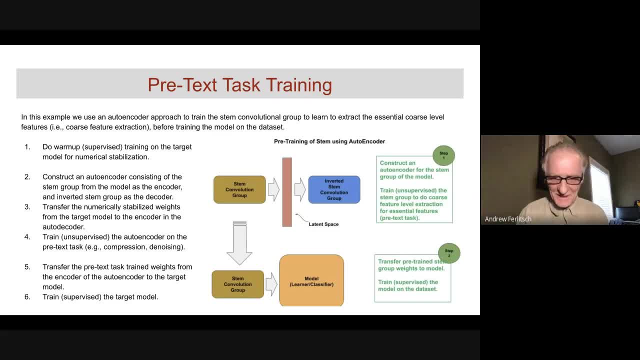 So I know this is a really busy slide here, So it starts like this: So we're going to take an existing model that we're going to do training- Okay, We've initialized the weights of it. We'll do warm-up training. If you're not familiar with that, we'll be discussing that in a 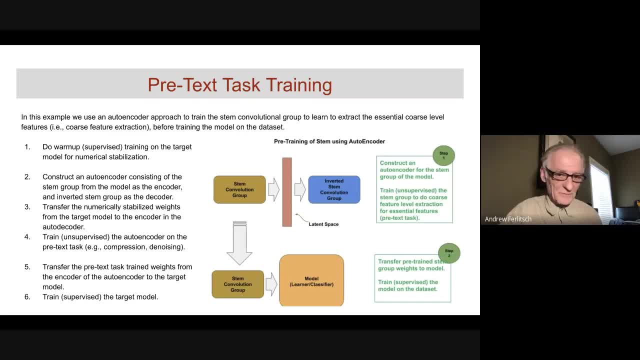 subsequent session. But the purpose of the warm-up training is to get numerical stabilization of those initial weights, And we do it in a supervised fashion. Now we're going to construct an autoencoder And what we're going to do is we're in a sense on that other model, we're 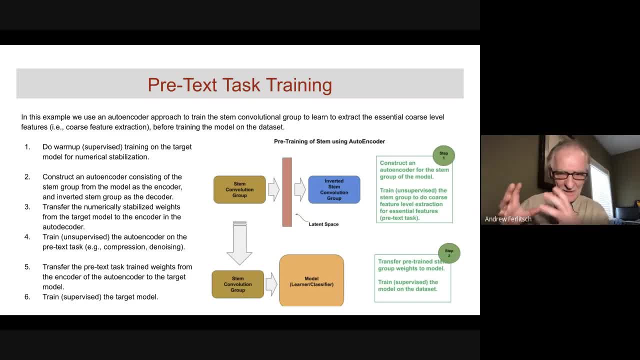 going to tear off the stem. Okay, Meaning we're going to just take the stem layers and the weights on the stem layers at the time we completed our numerical stabilization, And then we're going to make an inverted version of that stem. We're just going to reverse the layers the other way And 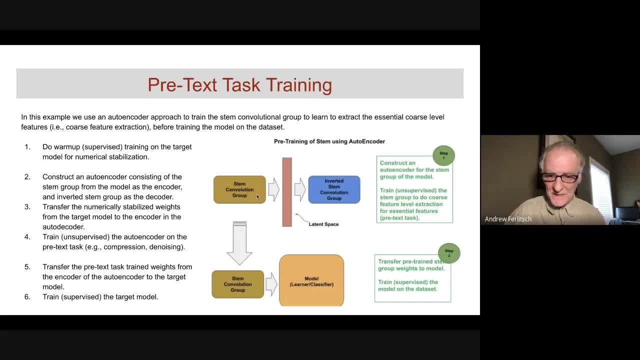 then we're going to tie them together where we have a latent space. So this stem convolutional group, like any stem, does that first, And then we're going to take the weights on the layers, first course level of feature extraction, But it also does pooling, And we're going to take 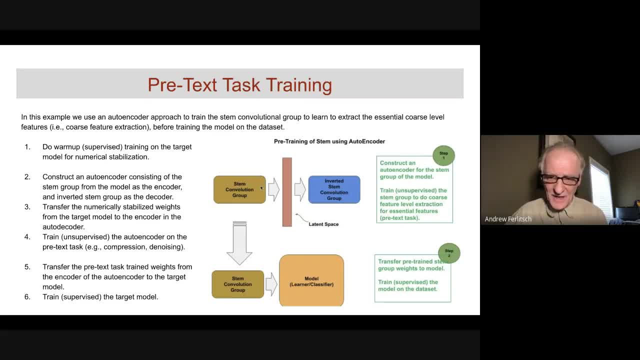 advantage of that. So we're going to then do unsupervised training here, typically with the identity function, so that this stem learns the optimal way of extracting the course level features where there are just simply the essential features. After we're done with this and we're 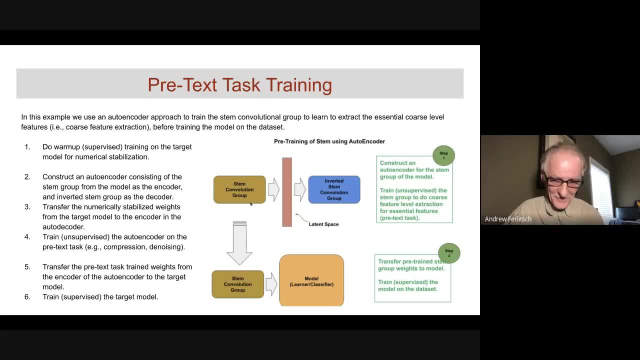 happy. we then take this now And then we're going to further train stem And we attach it back to our original model And then we do the final supervised training. And that's really it for pretext training. I have a little bit of 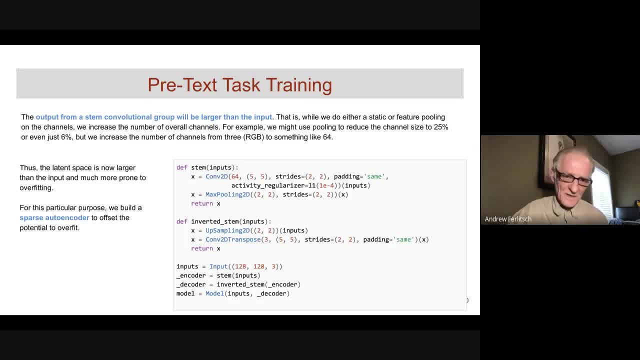 code here just to show you what it would look like. to wrap it up, So let's say: this is the stem from our model. Okay, It's going to have 64 filters. It does feature pooling already. Then there's max pooling, which does further pooling, And then we're going to take the weights and we're going to 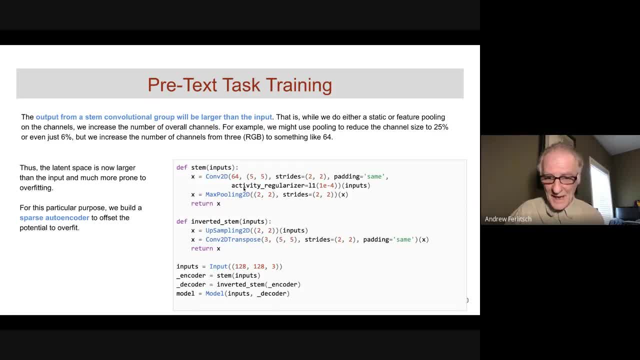 add this, Since this is the only convolutional layer, we're going to add the regularizer for the latent space to this one. The inverted one is just the opposite. If you're not familiar with upsampling 2D, it's just the reverse of max pooling 2D. So this would a stride of two would. 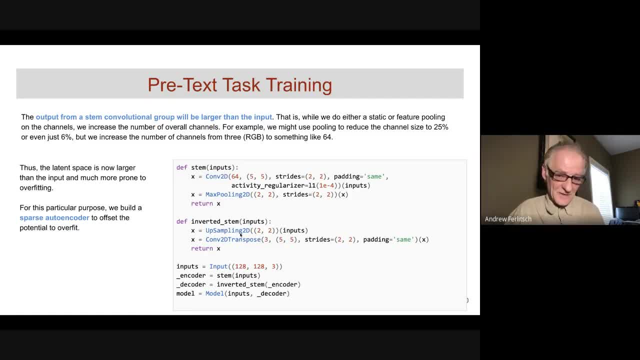 make it one half by one half, This would make it two times by two times. Then, of course, we're going to invert our convolution here with our transpose convolution. It's going to be strided, It's going to be unpooling. Okay, They have the same filter size here, five by five, But this time 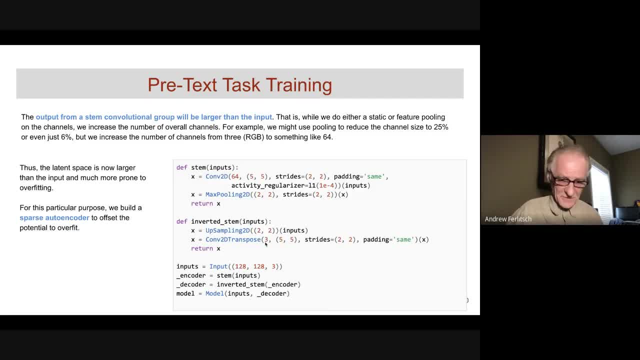 the number of output channels is three, so that we can reconstruct the image. And here we are. we create the input object. Hypothetically, we're going to say its shape is 128 by 128 three. We create the encoder right. Then we take the output from the stem and we use it as the input to the 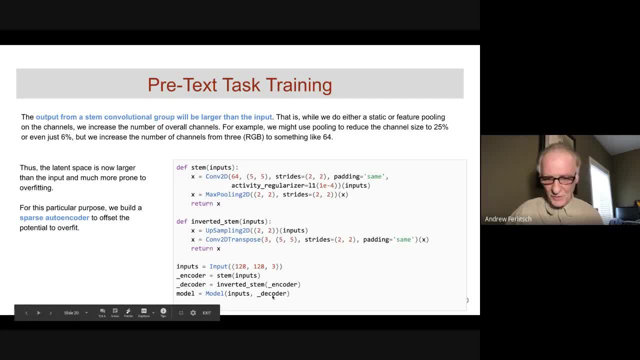 inverted stem. That's our decoder, And then we just pull it all together And that's our model, And that's all you need to do. Again, thank you for joining our session here.